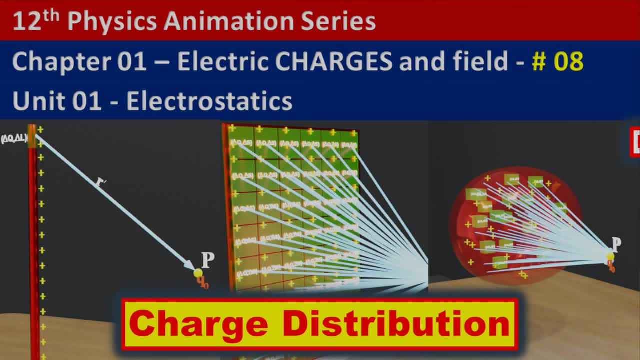 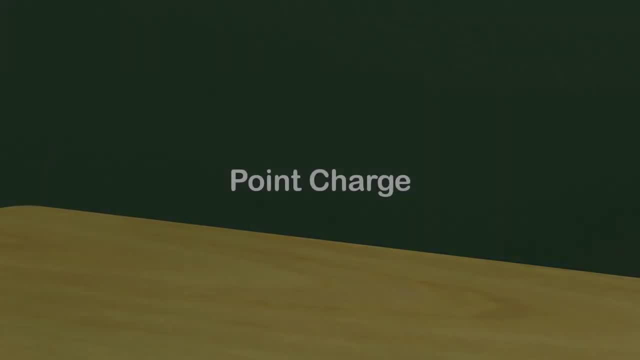 Hello friends, welcome back to physics and animation. So far, whenever we talked about the forces or electric fields between charges, we have considered charges as a point charge. But what if we want to determine the intensity of the electric field at a point due to charged wire? Because Coulomb's law is only valid for point charges. 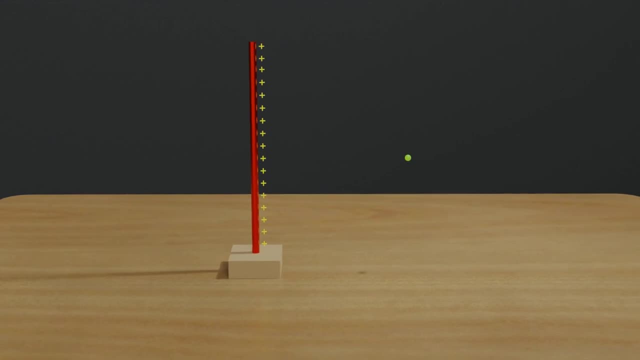 so we cannot apply it for charged wire. So let's start by understanding charge distribution. What is charge distribution? If we talk about the distribution of charges at microscopic level, we can have many charges on a wire And we can even think about spaces. 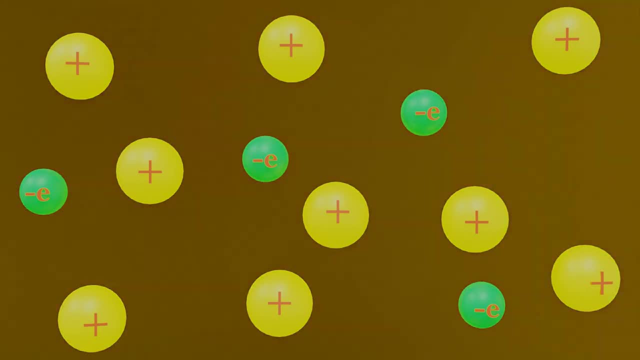 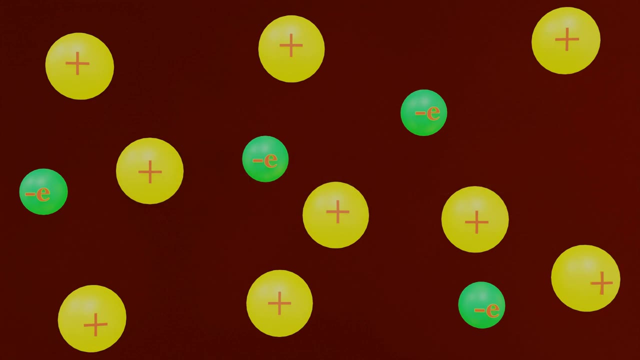 between charges where no charge is present. Such a distribution of charges is called a discontinuous charge distribution. At microscopic level, when we are dealing with few tens or hundreds of charges, it may seem possible to calculate resulting force and electric field intensity By adding up the force and electric field due to each individual charge for a point. 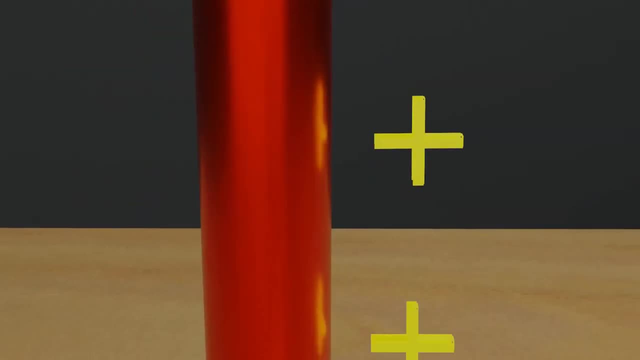 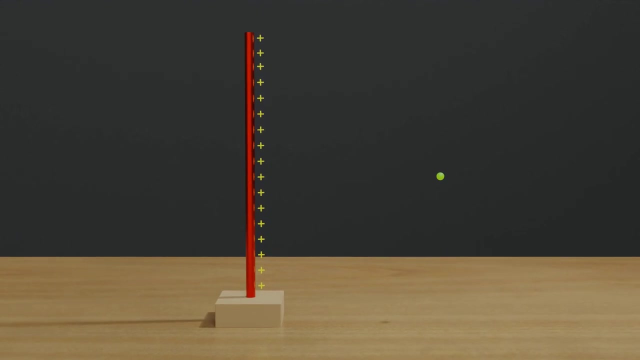 However, when we come to the macroscopic level where we have to deal with the countless charges in a wire, it becomes impractical to consider a discontinuous charge distribution Here. we require a continuous charge distribution according to which we assume that charges. 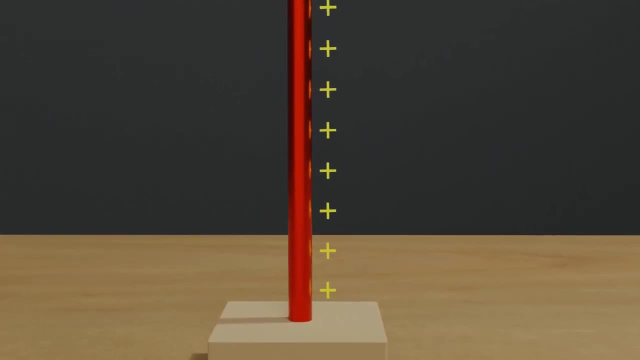 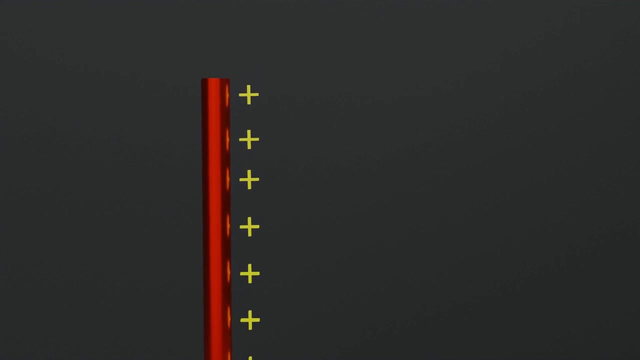 are present everywhere in the body and there is no gap between them. In other words, we assume that charges are continuously distributed throughout the body. Okay, if it is so, we can consider a small element del L on a wire. This element may be quite small. 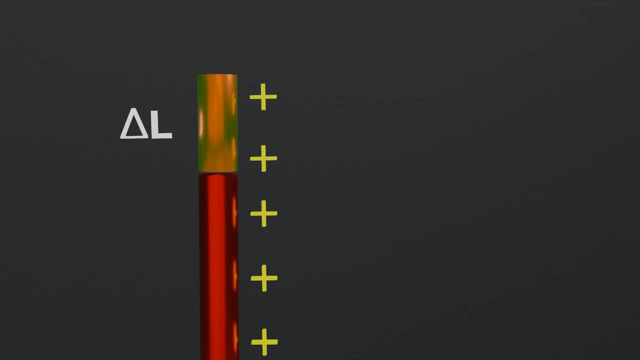 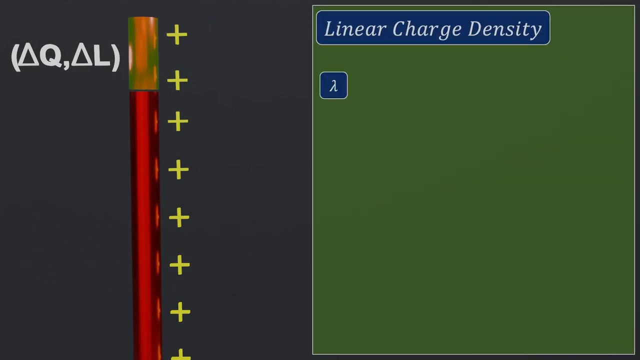 at the macroscopic level, but it would have a large number of charges on it, which is sufficient to define the charge del Q on the element. To simplify the calculation, a new term, linear charge density lambda, is introduced, which is equal to. 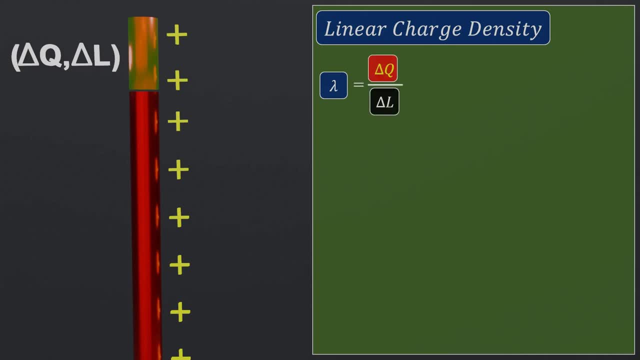 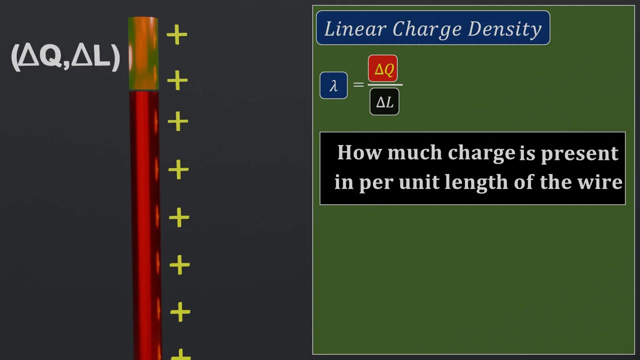 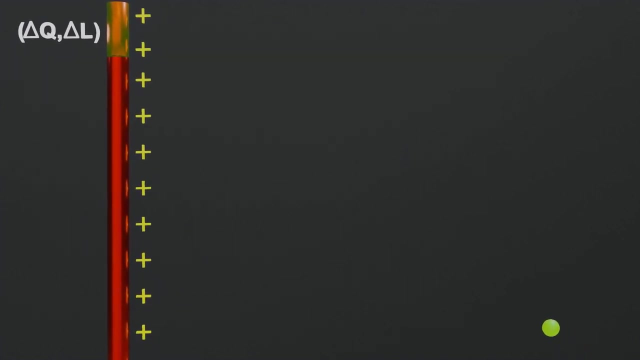 the charge del Q by del L. Linear charge density physically defines that how much charge is present per unit length of the wire, And this type of charge distribution is also known as Linear charge distribution or line charge. Now let's place a test charge Q0 at point P, separated by distance r' from the element del L. 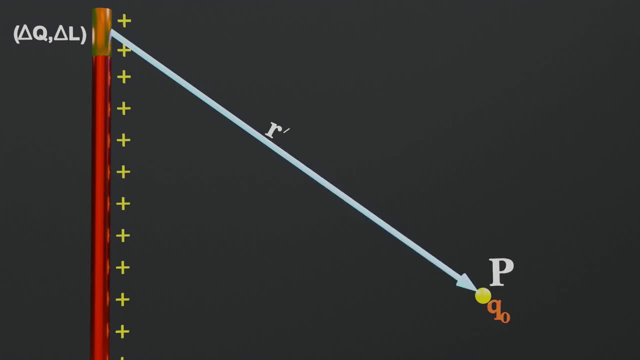 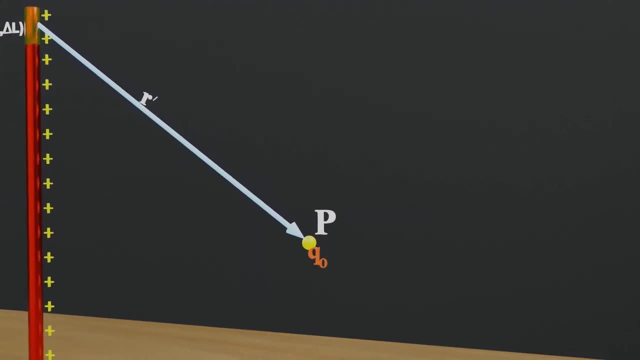 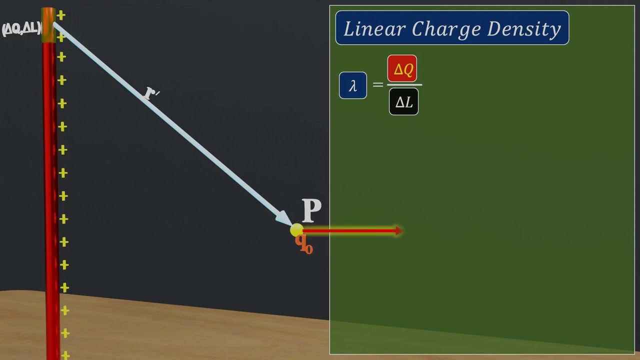 to measure the electric field intensity at point P. Since the size of the del L element is much smaller than the distance r dash, we can consider del Q as a point charge, and Coulomb's law can be applied now. Therefore, the small electric field del E at point P will be equal to one. 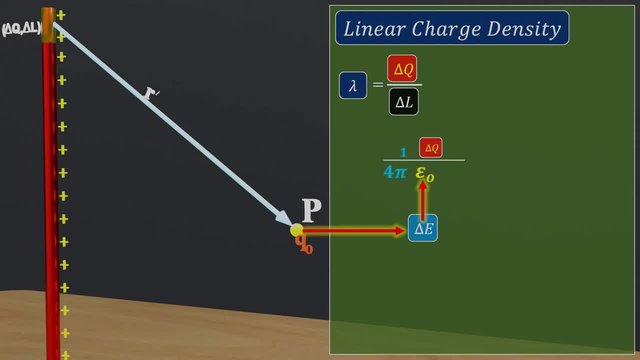 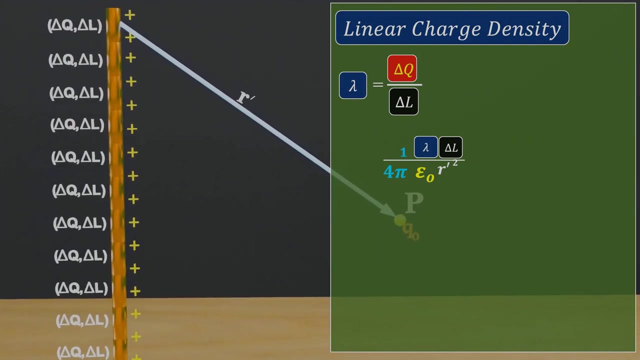 upon four pi epsilon naught times del Q divided by r dash square. Using the formula of linear charge density we can write the charge del Q as lambda into del L. In the same way we can consider a number of possible del L elements on the wire And. 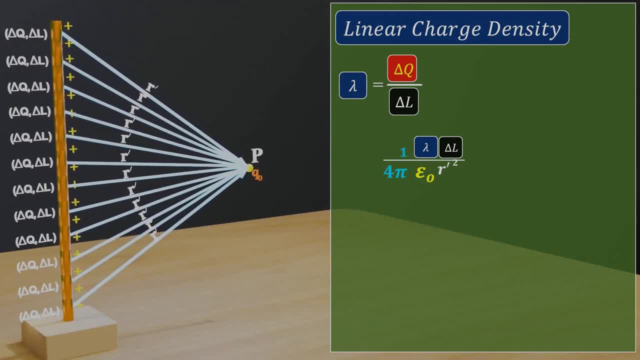 by using vector sum and the principle of superposition, we can calculate the total electric field at point P due to the all del Q charges. This can also be expressed in a simplified way, as electric field equals one upon four pi, epsilon naught the summation all del L lambda. 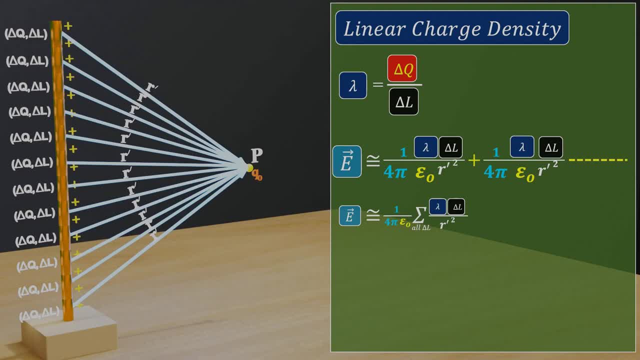 into del L divided by r dash square. Since electric field is a vector quantity, we need to multiply the equation with the unit vector r dash cap to specify the direction, As we saw in the last video, if we multiply the electric field equation with test charge. 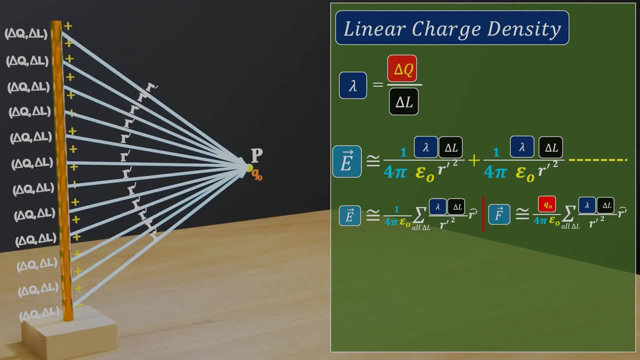 Q naught, we got the equation for the total force acting on Q naught at point P, due to the electric field. Ok, now, when del L is very small or tends to zero, the sum becomes an integral and we can write the equation for electric field and force in integral form. 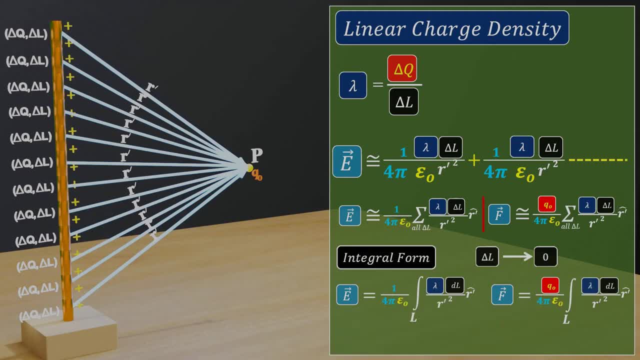 where del L is equal to one upon four pi epsilon naught divided by r dash square. So we can write the equation for electric field, as del L will be replaced by del. This is useful when we need to calculate the equation for electric field at a point due. 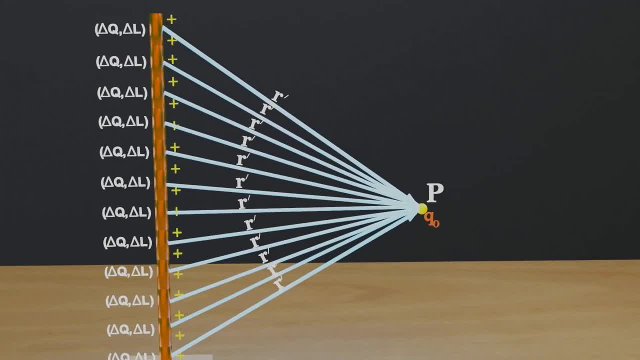 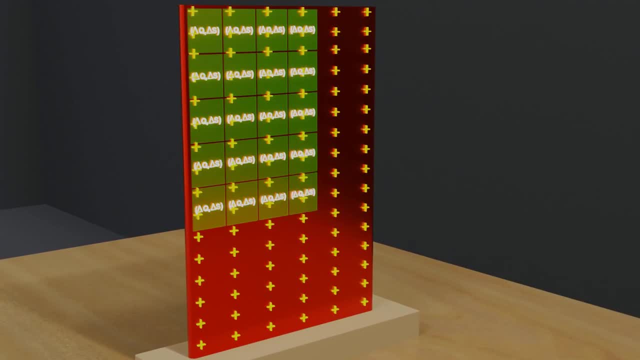 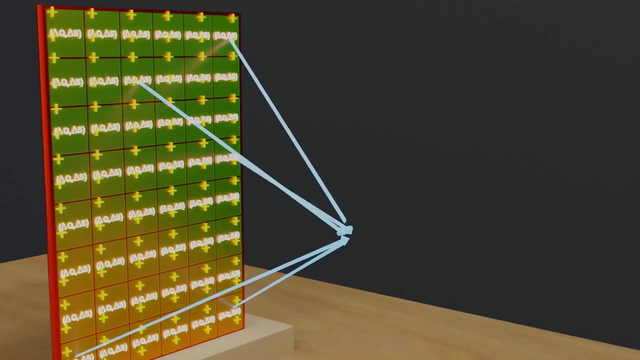 to a wire or line charge. Similarly, if we are given a surface charge distribution, we can take multiple small surface elements del S and del Q and use the superposition principle to calculate the electric field intensity at point P, just as we did for the wire Just.